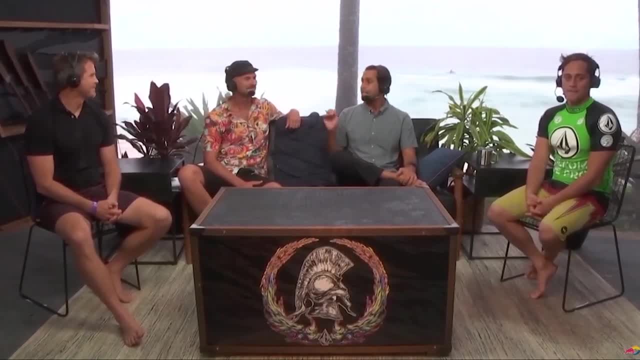 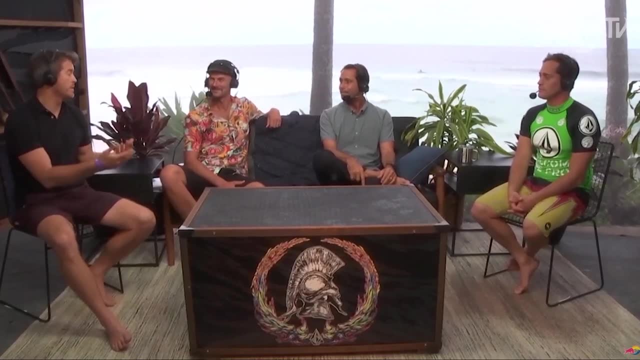 so you can get those extended forecasts And the forecast analysts too, those premium analysts that you can get. Yeah, we try and break things down and really do what I'm doing here and what I do for Volcom and Marty. Speaking of breaking it down, Kevin, let's break this down. 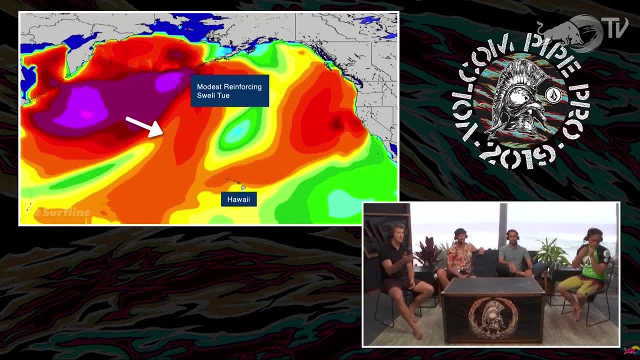 We've got the forecast on the screen, some of the models, Yeah. so we've got a lot of activity in the western Pacific and that's what sent the swell today. It's going to get a little smaller the next couple of days. 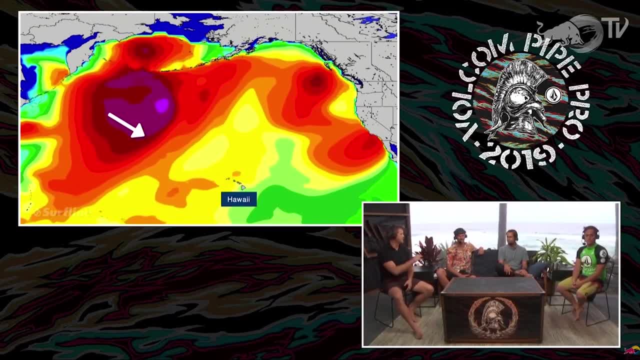 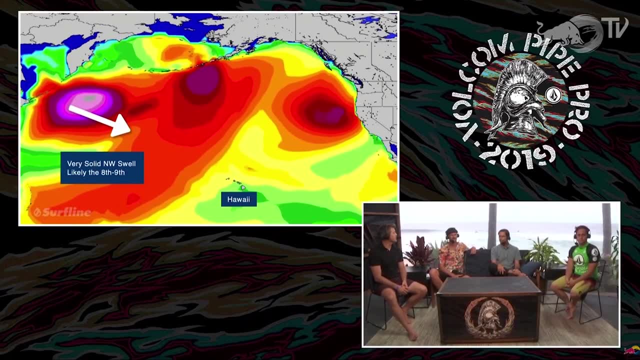 but we have another pretty good-sized swell on Wednesday. So the size of the surf that we saw this morning, I think that's what we'll more consistently see throughout the day, And right now wind looks pretty good on Wednesday too- Really light in the morning, maybe like perfect wind in the morning. 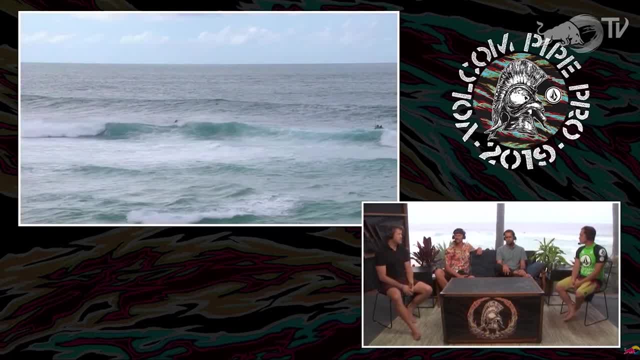 and then kind of getting swirly and kind of light variable in the afternoon. A bunch more swell towards the end of the week, but it looks like poor wind right now. It looks like north wind will probably start to kick in sometime on Thursday. 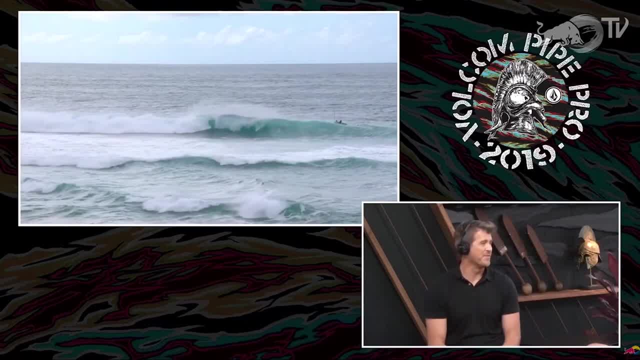 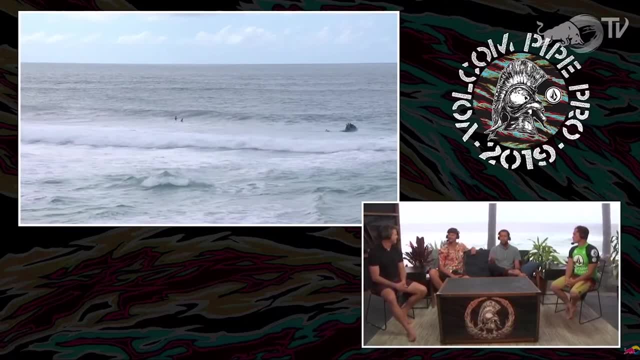 and then we're just kind of in for another north wind session for gosh. a week, 10 days, Kind of like what we just saw. so cool and windy, Cool, windy north winds. Pick your spots, everyone on the islands. 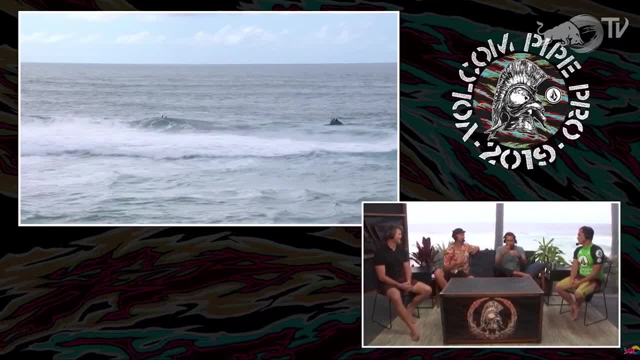 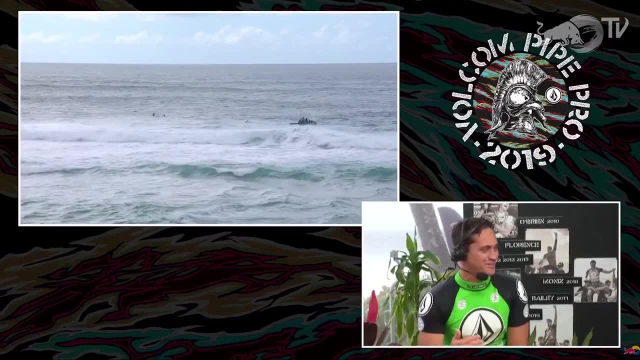 You guys all know the north wind spots. It's an island, right, Kevin? do you practice that voice? Your voice is so consistent Every time I ever heard you speak. you've got the perfect voice for TV and forecasting and everything. 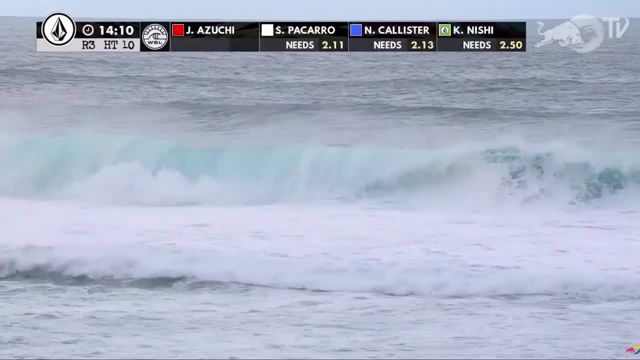 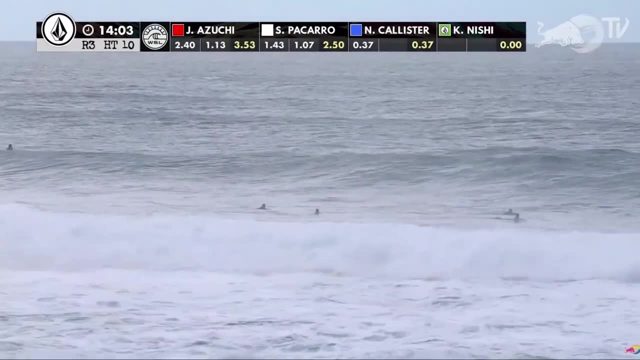 It's like the professional voice kicks in right now, Now that we have no takers on this. we can talk about sets here and we can talk about swell periods. There's been a lot of talk about the period of the swell, in which favors either the lefts or the rights. 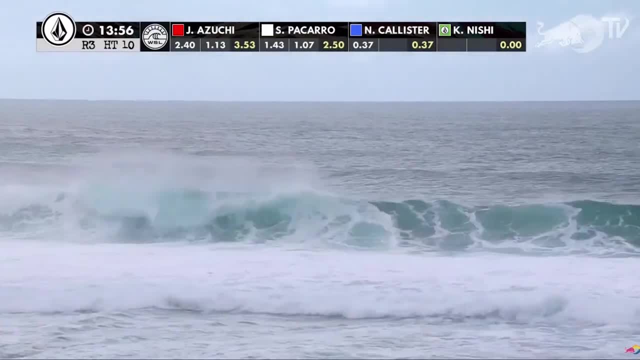 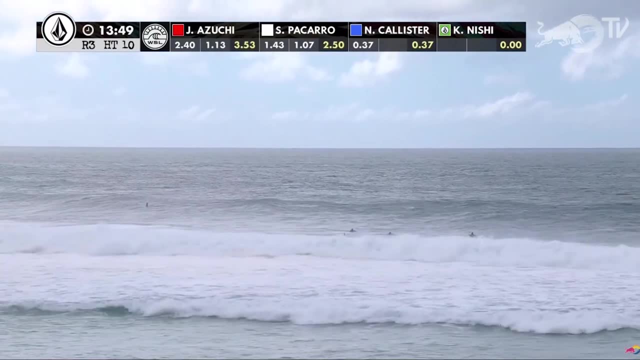 Can you explain? Can you explain swell period to our audience first of all? Sure, So swell period is the time it takes two successive waves to pass a stationary point. So that could be a buoy, It could be a jetty, It could be a rock. 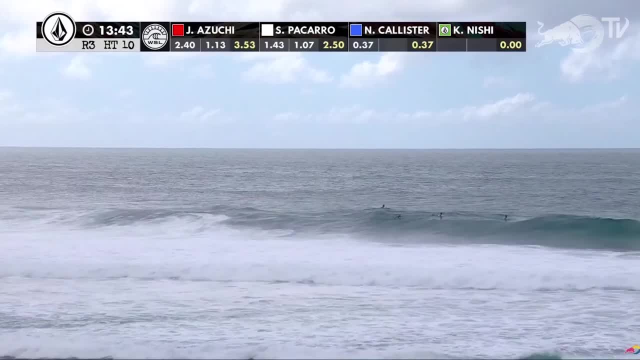 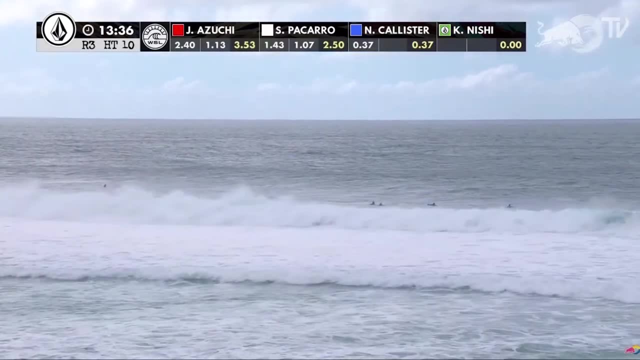 And we measure that in seconds. And swell period is really important for us for forecasting because it determines not only how quickly a swell might travel from a storm to where we are- because longer period swells travel faster than shorter period swells- but also how big the waves might be once they arrive here.